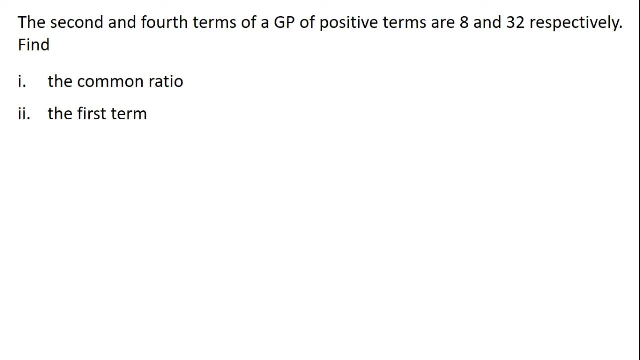 Find i the common ratio, ii, the first term. We have learnt that the value of a term in a GP is denoted by un and un is given by the formula a, r exponent n minus 1, where a is the first term of the GP, r is the common ratio and n is the number of the term whose value we want to find. The common ratio of a GP is denoted by un and un is given by the formula a- r exponent n minus 1.. The common ratio of a GP is denoted by un and un is given by the formula a r exponent n minus 1.. 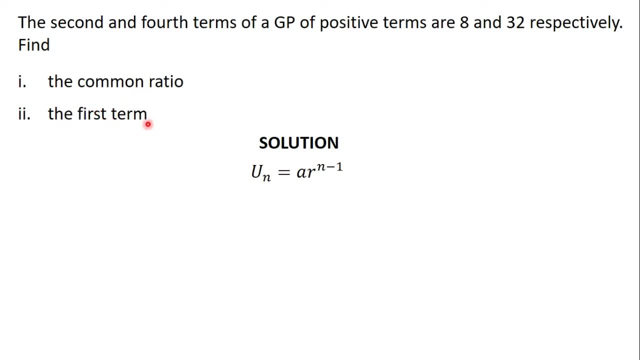 The common ratio of a GP is denoted by un and un is given by the formula a- r exponent n minus 1.. The common ratio of a GP is denoted by the formula a- r, exponent n minus 1.. question wants us to find the common ratio and the first term. so we are looking for a and r. 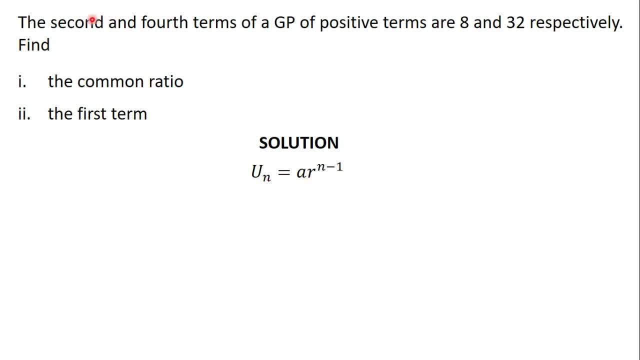 from the question. we are being told that the second term and the fourth term are 8 and 32 respectively, meaning that the second term of the gp is 8. the second term of the gp will be denoted by u2, so u2 is equal to 8. since the second term is 8, we are talking about the second term, so the 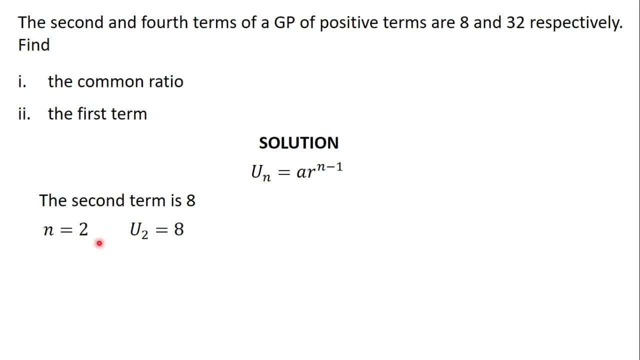 number of the term is 2, so it means that n is equal to 2. let's find u2 from the formula. from the formula, u2 will be equal to a r exponent, 2 minus 1, since n is equal to 2. so we have u2 is. 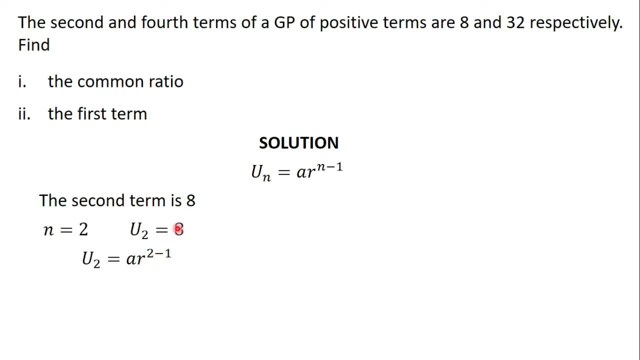 equal to a r exponent 2 minus 1. we know that u2 is equal to 8, so we can replace u2 here with 8 and we will have 8 is equal to a r, since 2 minus 1 will give us 1 and r exponent 1 is the same as r. so 8 is equal to a r. we have a r. 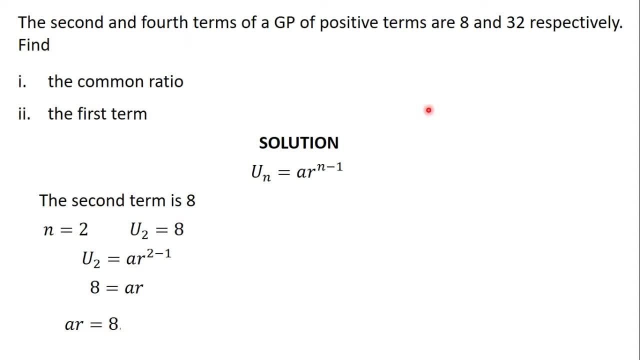 is equal to 8. we also know that the fourth term of the gp is 32. the fourth term will be denoted by u4. so u4 is equal to a r exponent 2 minus 1. so we have a r exponent 2 minus 1 since the second. 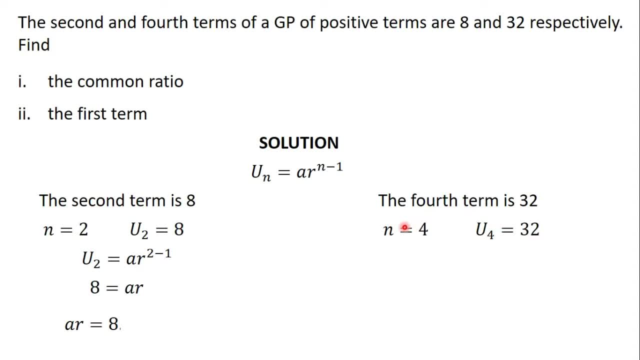 term is similar and we will bequeave a third term to a r exponent 2 minus 1, since the fourth term is equal to 4. so we have a r exponent 2 minus a r-2, since the first is equal to the third term. 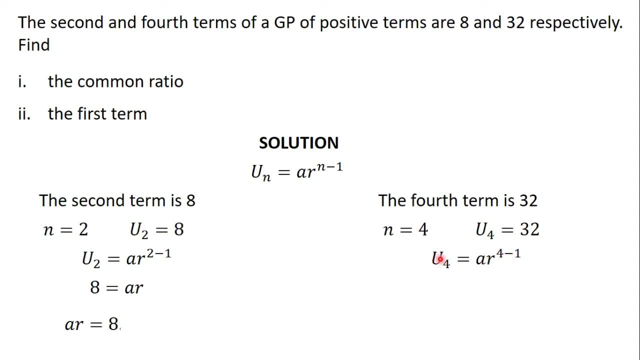 we are talking about the fourth term, so the number of this term is 4, so n is equal to 4. let's find u4 from the formula. from the formula, u4 will be equal to ar exponent 4 minus 1. u4, rootsete to you, so we have 32- is equal to a r exponent 3, since for minus one give us three, so we: 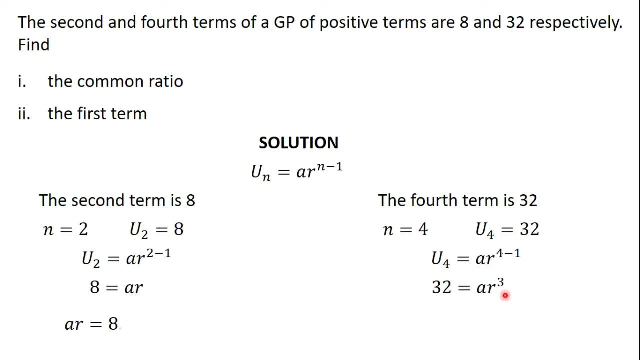 have 32. we will base our synthesis pena infront of the formula. so if we find that u2 is equal to 4 is equal to a r exponent 3, this can also be written as a r exponent 3 is equal to 32. so we have two equations here and two variables. i'll call the first one equation 1 and the second. 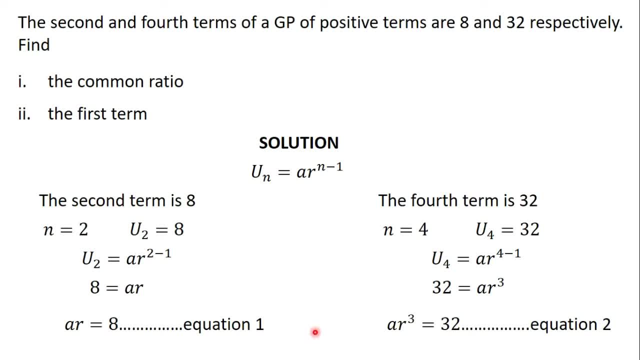 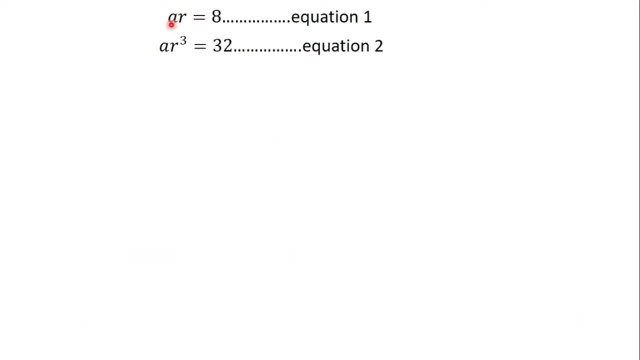 one, equation 2. we have two equations, two variables, so we can solve these equations simultaneously. once again. equation 1 is a r is equal to 8 and equation 2 is a r exponent 3 is equal to 32. i want to eliminate a from these two equations. in the first equation, a and r are multiplying. 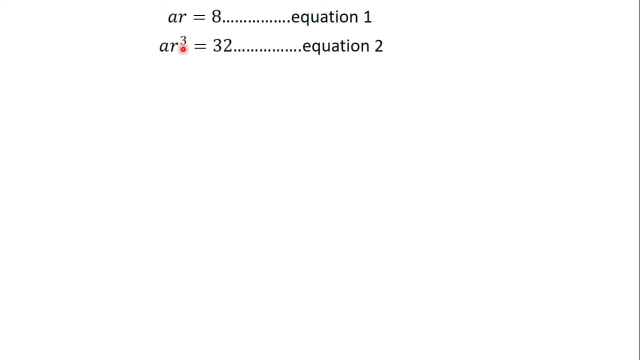 in the second equation, a and r, exponent 3 are also multiplying. because we have multiplication in both equations, i'm going to divide the equation by the number of variables. so i'm going to divide one equation by the other in order to eliminate a. so i'm going 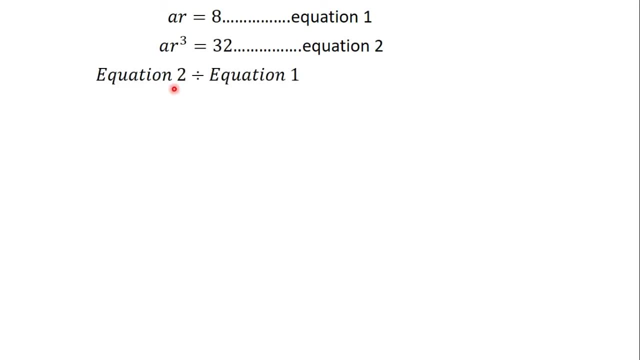 to divide equation 2 by equation 1. equation 2 divided by equation 1, i'll take the term on the left hand side of equation 2, which is a r, exponent 3, and divide it by the term on the left hand side of equation 1, which is a r, and this will be equal to. then i'll 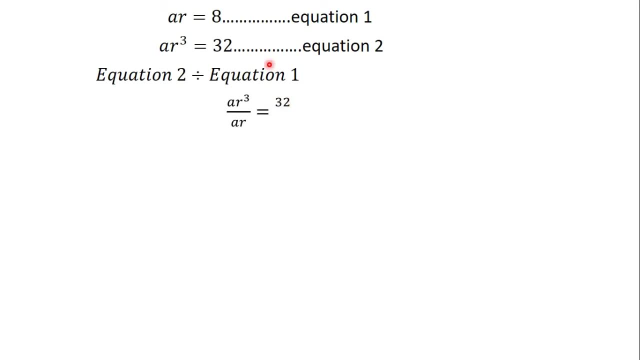 take the term on the right hand side of equation 2, which is 32, and divide it by the term on the right hand side of equation 1, which is 8, so we have a r exponent 3 divided by a. r is equal to 32 divided by 8. we know that in this case a will cancel a. so on the left hand side we are going to. 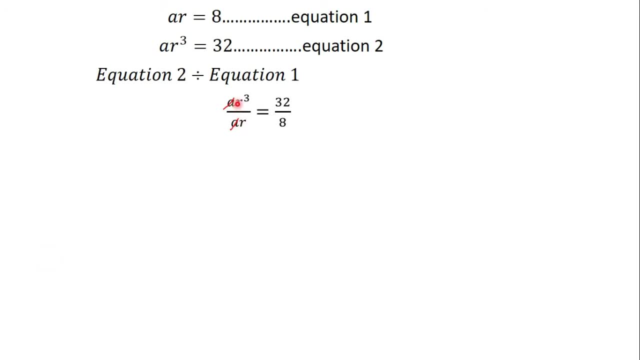 have. on the left hand side we are going to have r exponent 3 divided by r, and on the right hand side you have 32 divided by 8. from indices we learnt that r exponent 3 divided by r is equal to r exponent 2. 32 divided by 8 is equal to 4. so we have r squared, or r exponent 2 is equal to 4. 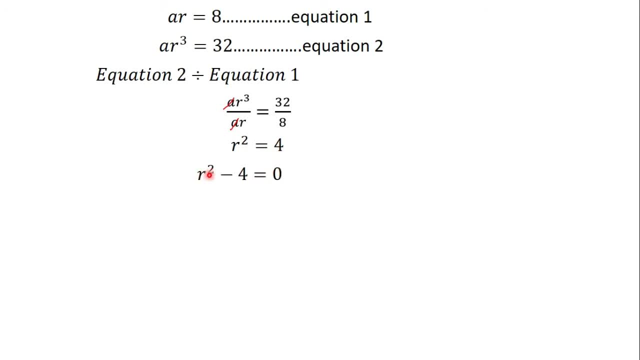 we can rearrange this as r exponent 2 minus 4 is equal to 0. 4 can be expressed in index form as 2 2 2. so we have r squared minus 2. exponent 2 is equal to 0. from algebra we can see that this: 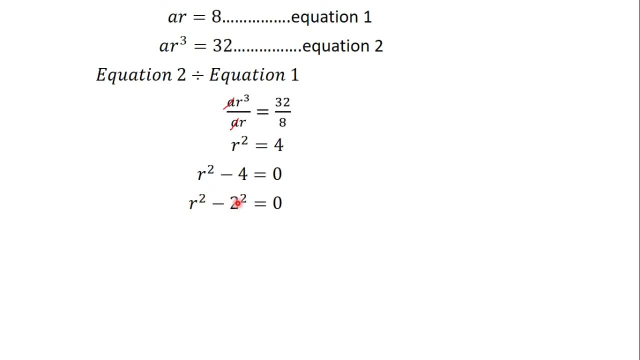 expression on the left hand side, r squared minus s? squared, is a difference of two squares. in the videos on difference of two squares, we learnt that an expression of this form, that is, r squared minus 2 squared, can be expanded as r minus 2 in one bracket. 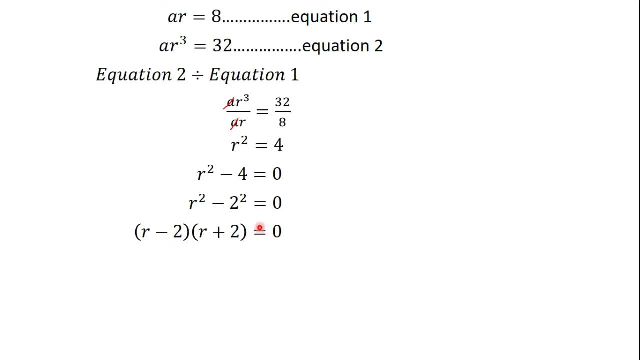 then r plus 2 in another bracket. i explain this into details in the videos on difference of two squares and the algebra. so if you want more information about difference of two squares, watch the video on difference of two squares and the algebra. let's continue with our solution. we have learned that when you have an equation like this in order 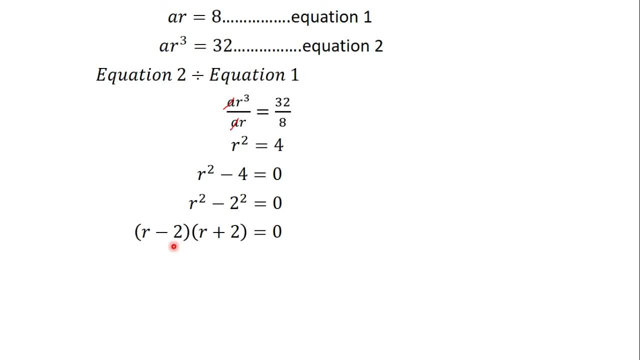 to find the values of r. you equate the content of the first brackets to zero. then you calculate the data of the two brackets to zero. then you calculate the value of the two brackets to zero, then you you equate the content of the second bracket, also to zero. so for the first bracket we have r minus. 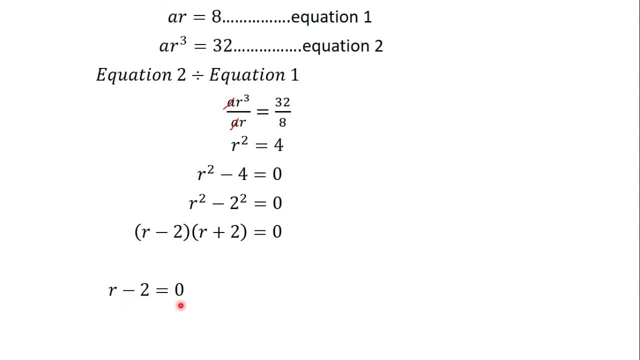 two, so you equate that to zero. so we have r minus two is equal to zero, and this will give us r is equal to two. you do the same thing for the second bracket. we have r plus two, so you equate that one also to zero. we have r plus two is equal to zero and r is equal to minus two. so you can see that. 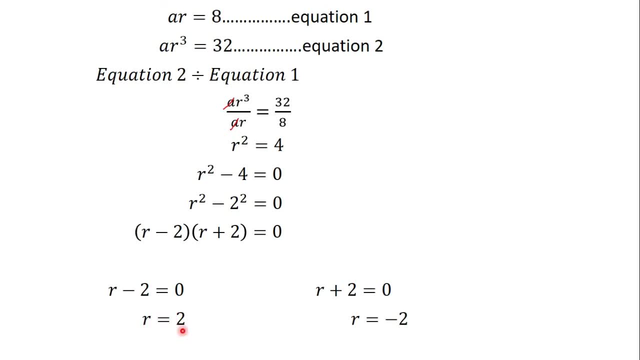 from here. we have two values of r. r is equal to 2 and r is equal to minus 2. but remember that in the question we were told that the gp has positive values only. that means that all the terms in the gp are positive. if all the terms in the gp are positive, then it means that the common 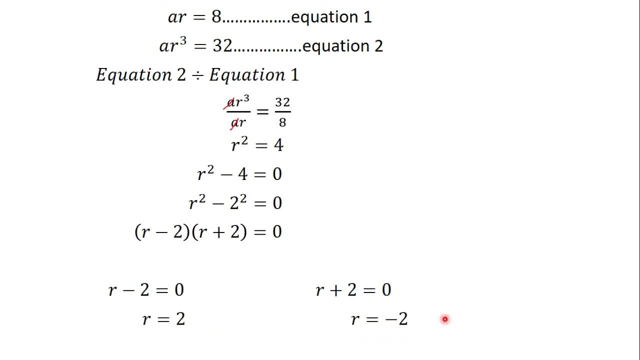 ratio should be positive, because if the common ratio is negative, then some of the terms will be negative. we know that from the question. all the terms in the gp are positive. so because all the terms in the gp are positive, then it means that we are going to pick the positive value of r. 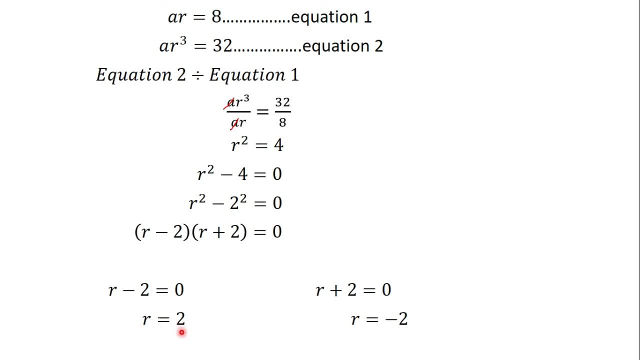 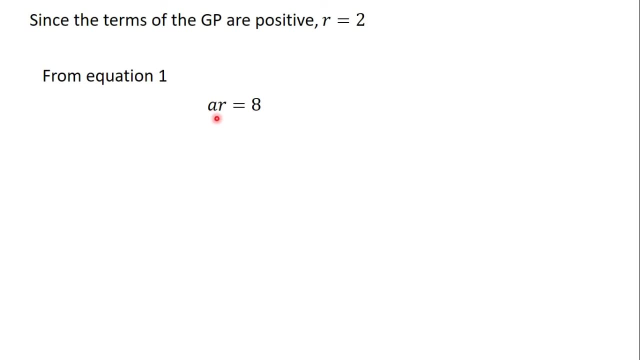 is equal to 2.. From equation 1, we know that AR is equal to 8.. So if R is equal to 2, then we will have A times 2 is equal to 8.. This will give us 2A is equal to 8.. So we divide the left-hand side. 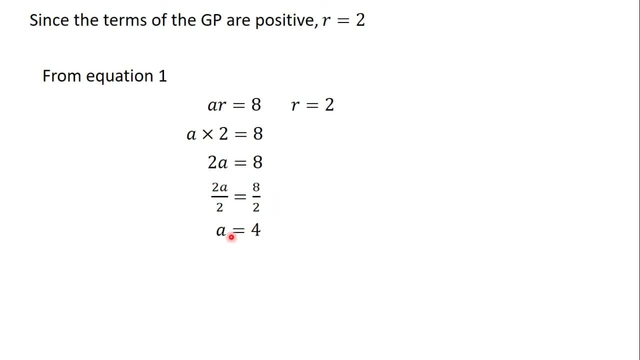 by 2,, we divide the right-hand side by 2, and A will give us 4.. Remember that R is the common ratio of the GP and A is the first term. We have found R to be 2 and A to be 4.. So we can say that. 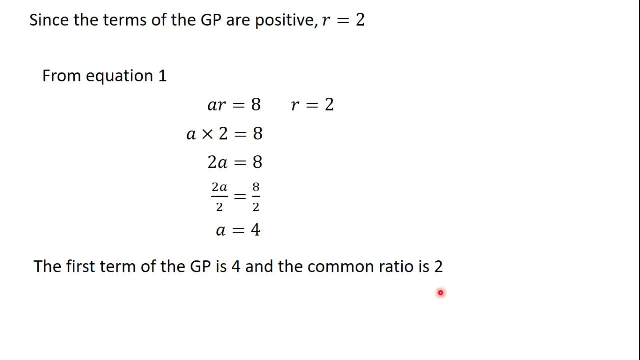 the first term of the GP is 4 and the common ratio is 2.. Thank you for watching this video. Subscribe to this channel for more videos. In the next video, we are going to solve another question on finding the common ratio of a GP. Bye-bye. 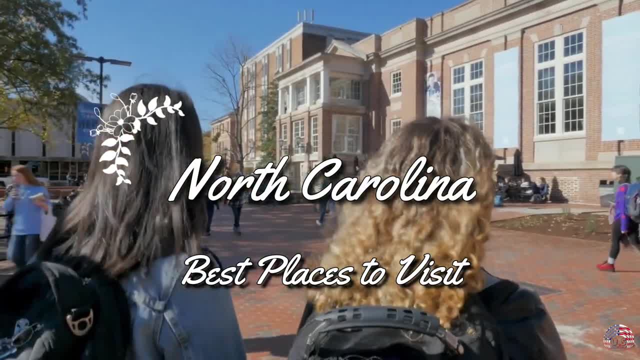 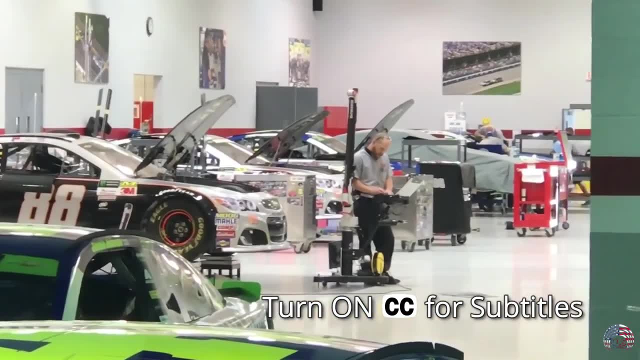 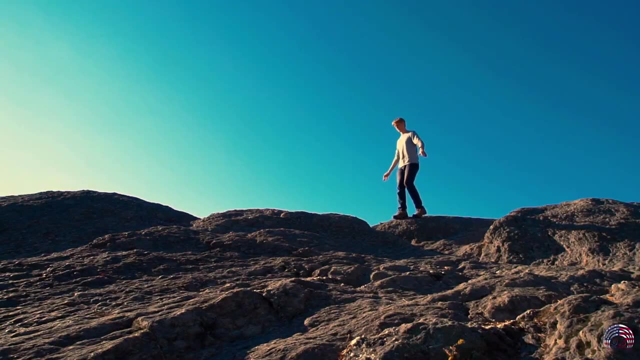 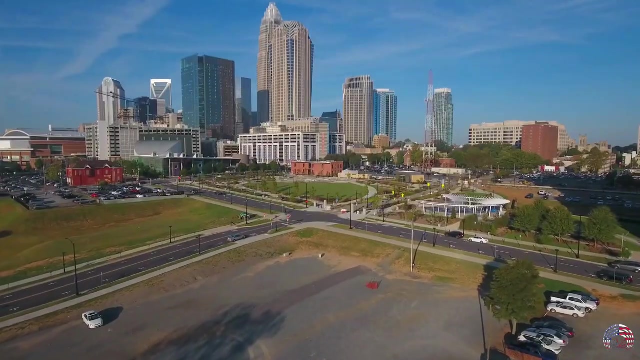 North Carolina truly has something to offer everyone, with stunning beaches, breathtaking mountains, Old South Charm and the official home of NASCAR, the world's most watched spectator. sport Visitors can take part in outdoor activities like mountain climbing, hiking, skiing and an experience of Appalachian culture in the Blue Ridge and Smoky Mountains, or visit the diverse cities of North Carolina.